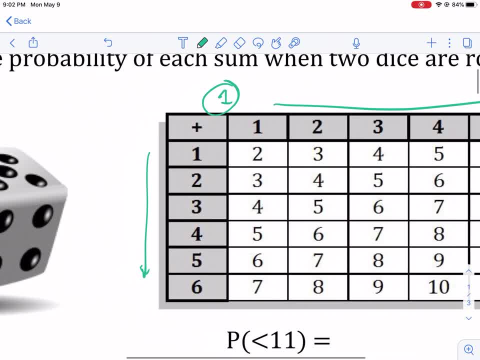 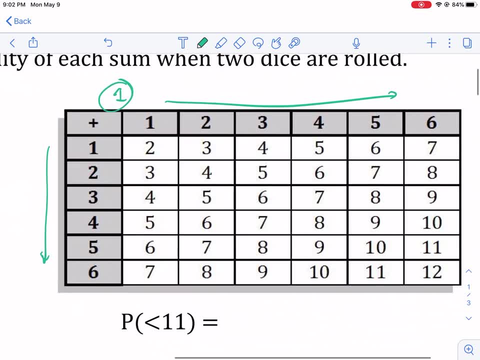 white, you're not going to see the number one, because that's impossible to roll a one when you have two dice and the minimum value on each dice is a number one. So the minimum value, of course, is two snake eyes, as you might hear it said, and the biggest is 12.. And then both of those. 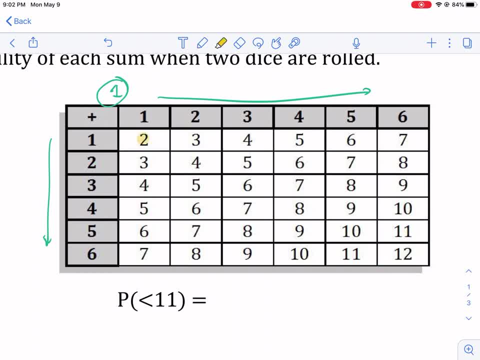 only happen one time. There's only one way to roll those two numbers. Okay, Now you'll see, the most popular number is seven, And that's why you see that the most number of times. it's the highest likelihood of rolling a seven, Cause there's the most. 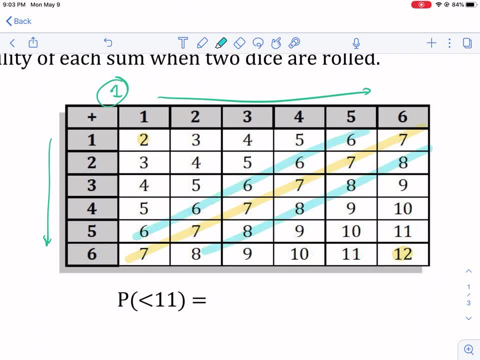 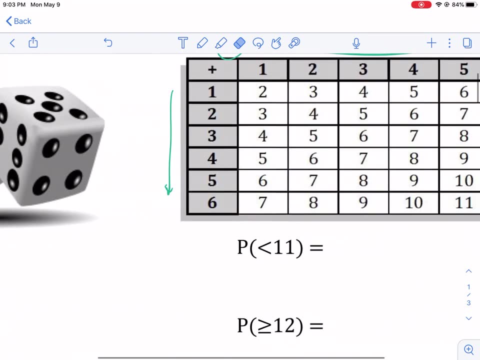 combinations to get a seven. Six is the next popular, along with eight. six and eight are tied, And then we have five and nine as also popular choices, And then it's a little bit more sparing after that. But the point that I'm getting at is we need to find bigger than two. So if we're 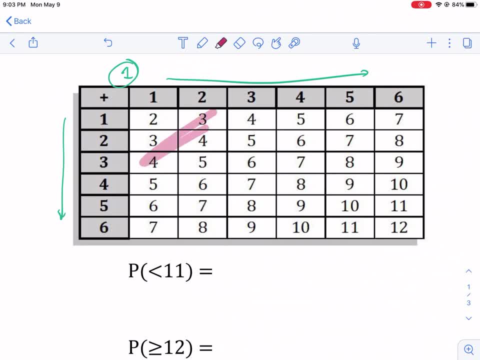 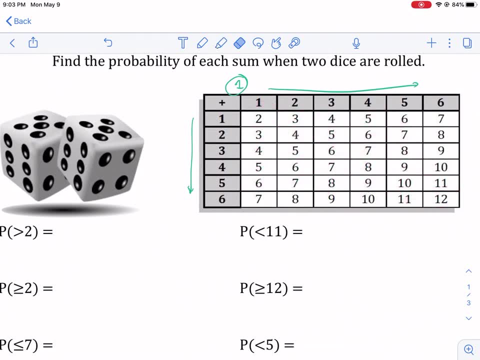 looking at this chart, here we're looking for all the numbers bigger than two. So that's all of these, and leaving this one out. So how do we do that? Well, if we look at this chart, we want to know the total number of. 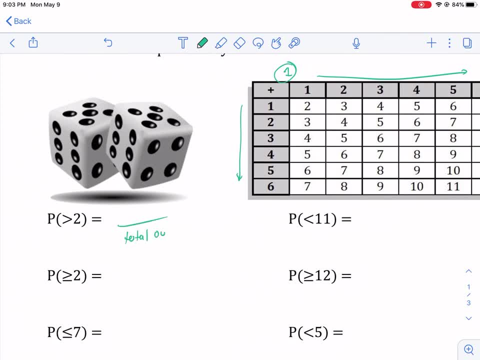 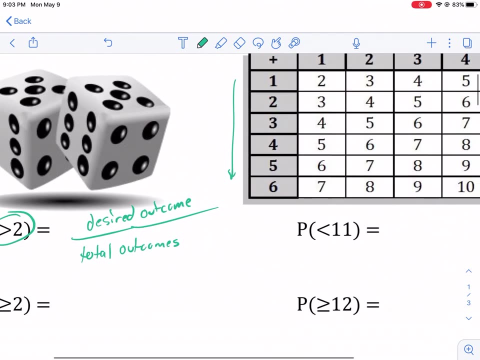 possible outcomes: Okay, So the total outcomes, but we only want the desired outcomes. Okay, And the desired outcome is the one that's in parentheses. So in this case, that's a terrible line. In this case, the desired outcome is in parentheses: something bigger than two. Well, 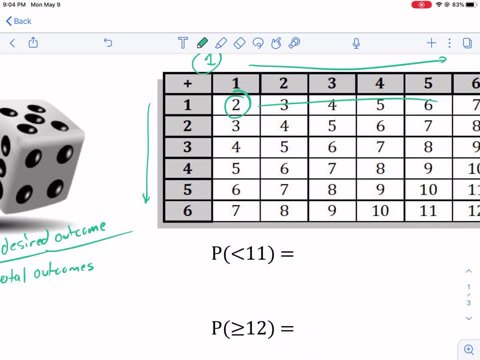 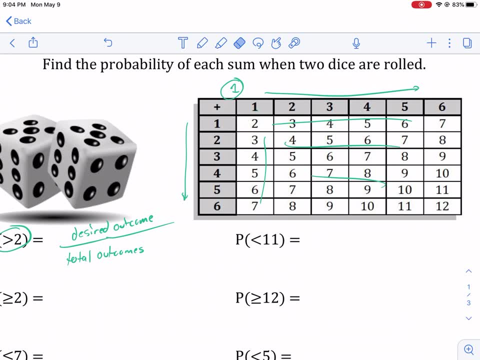 bigger than two. is everything this way, this way, this way. Okay, Basically the whole chart. So how many values, how many desired outcomes are there total? Well, we can count them, The total number of outcomes, And I don't like that for a highlighter: One, two, three, four, five, one. 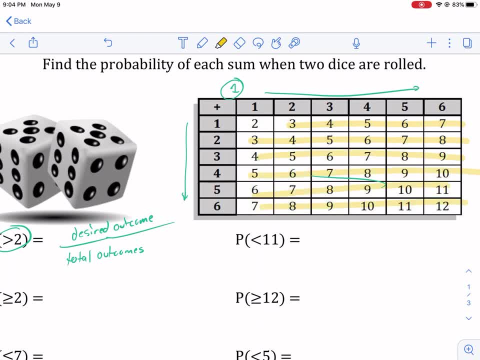 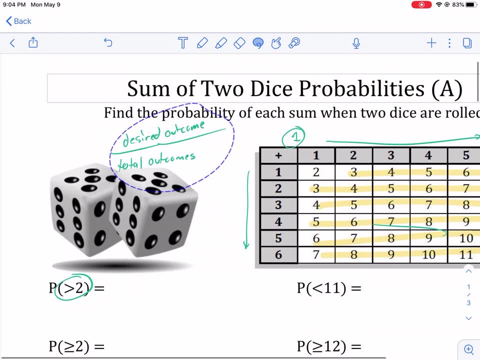 two, three, four, five, six- Okay, We can count all of these. The total number of desired outcomes is 35. So for this, my desired outcome, let me go ahead and move this over And I'm going to just 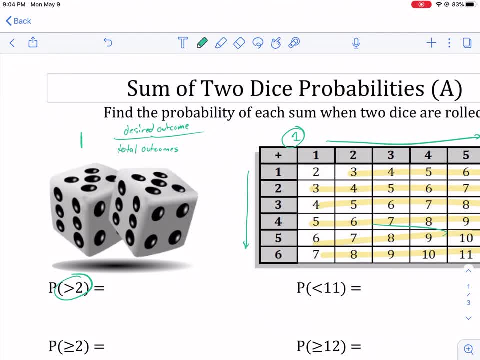 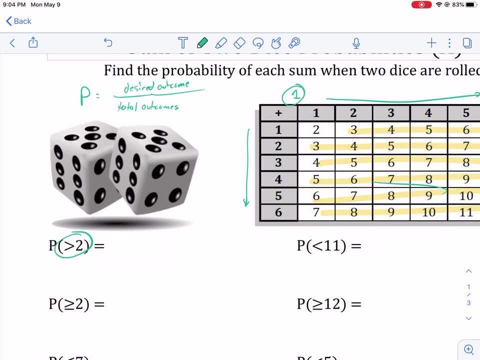 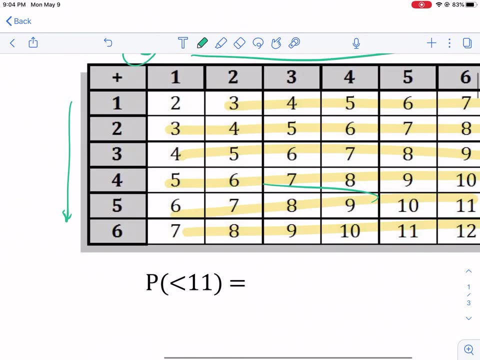 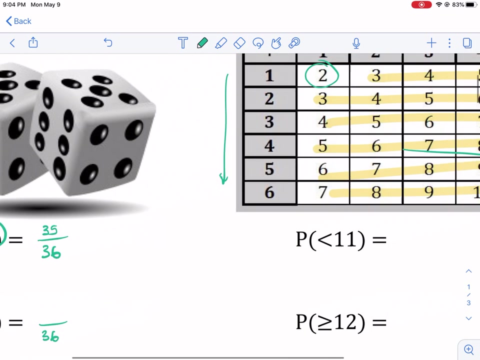 say this is equal to shrink, wrap it. That's probability. Okay, So probability is equal to desired outcomes divided by total outcomes. So my total outcomes for this one is 35. And my total outcomes again, I was everything except the two. So that just adds one more, That is 36.. And all of these are going to be out of 36.. Okay, 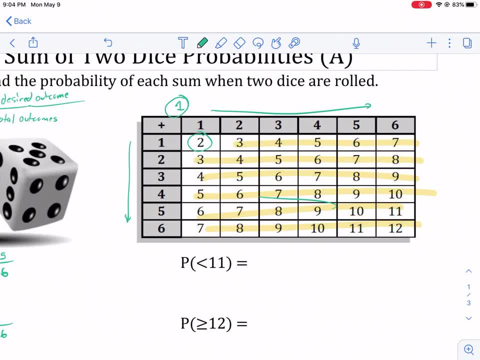 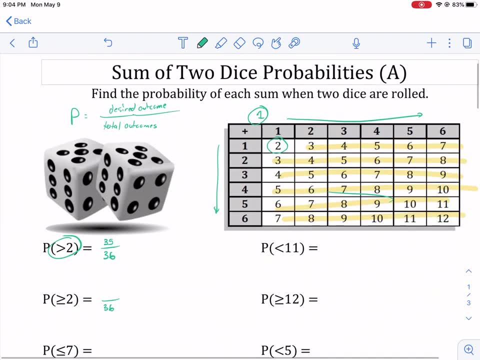 There's 36 possible combinations of dice that you can have: The one with the two, the one with the five, the one with the six, the three with the four, Okay, So I'm going to just add one more. Okay, You get the point. There's 36 possible combinations, So all of these are going to be. 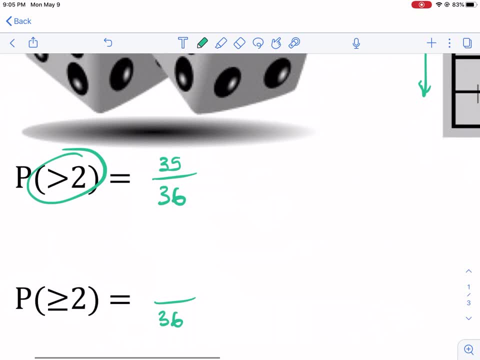 out of 36.. Okay, So this one is 35 out of 36.. So how do we find the probability? We just do division now. So we're going to do 35 divided by 36.. You can even do this on a calculator. 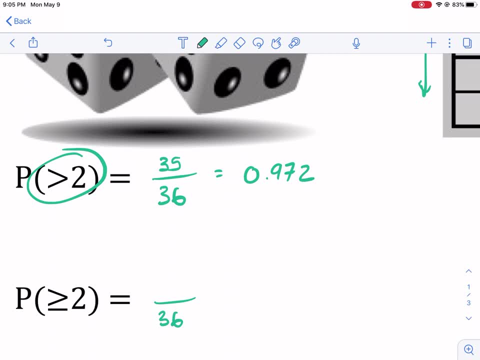 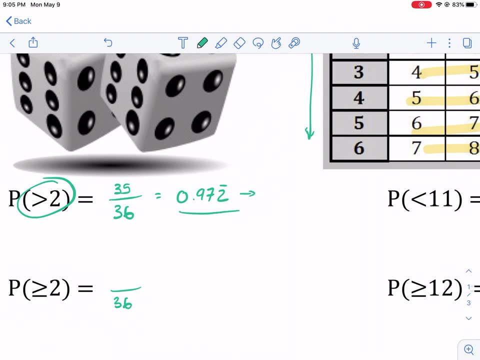 and I get 0.972.. And that's actually repeating. I'm going to round And I like doing it in terms of percentage. You don't have to like, technically that's good enough, Okay, But percentage wise, 97.2%. 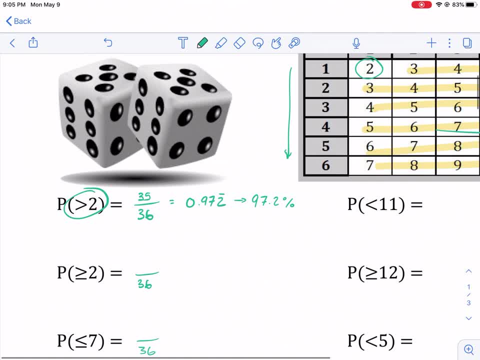 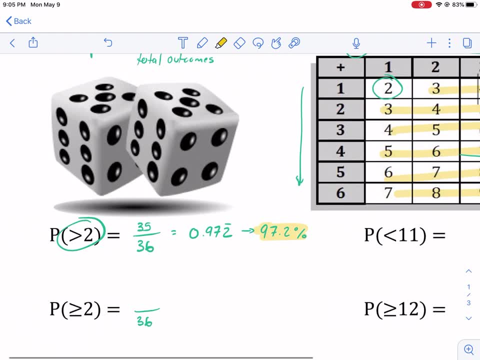 Okay. So if you're playing a game or you're doing a chance game, or you're at the county fair or whatever, and you want to know the probability of rolling a two- sorry, a three or bigger on that dice, you have a 97% chance of that happening. Now, of course, there's always a chance you do. 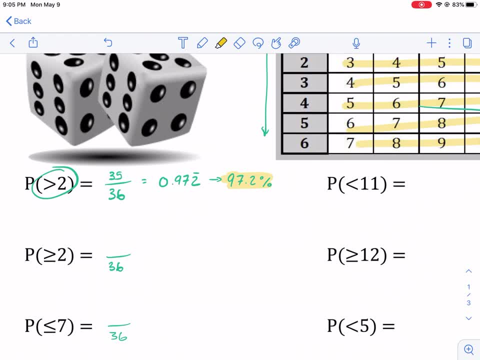 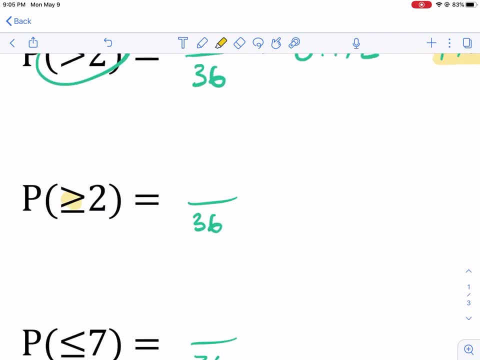 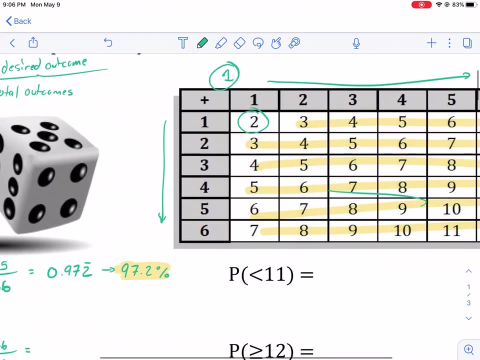 roll that two, but it's a. it's not very likely. it's it's less than three percent. Okay, Now let's go for two or greater. Okay, This is greater than or equal to two. Well, I hope you know that. it's 36 out of 36.. Okay, There's 36 options that are two or bigger. 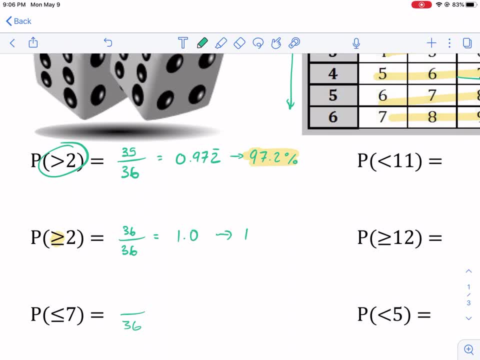 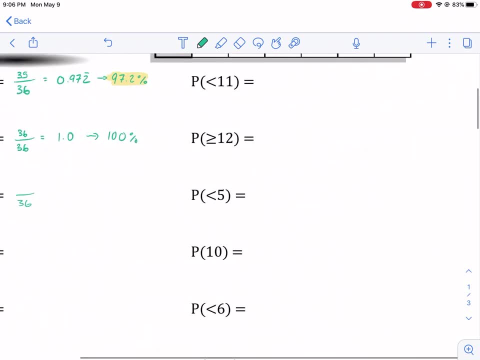 So that would be 1.0, 100%. You have a 100% chance of rolling a two or bigger, Okay, So that's all you're doing with these. is you're looking for these particular outcomes for this one, For example? 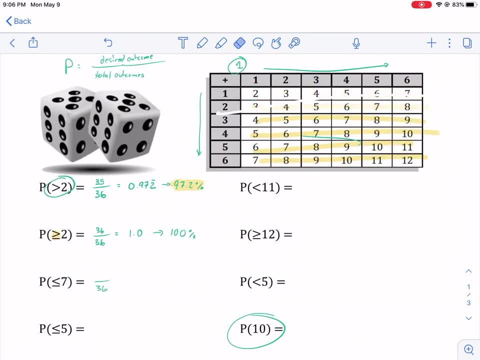 P10, we're going to look at the total number of tens that we have on here. Okay, So let me do some erasing real fast. So the total number of tens: one, two, three. we just have three, two. 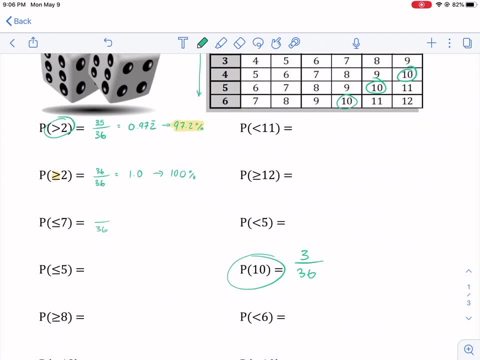 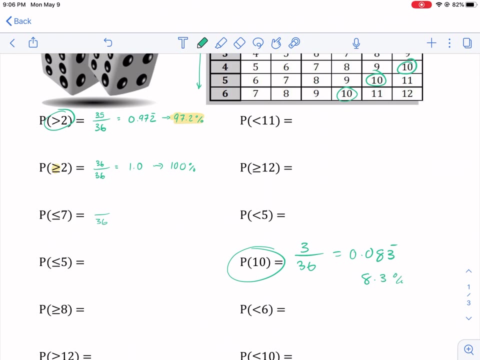 three tens, three out of 36.. So I'm going to go to my calculator: three divided by 36 and I get 0.083.. And that's actually repeating. If you want to do it as a percentage, 8.3%, Okay. And to get: 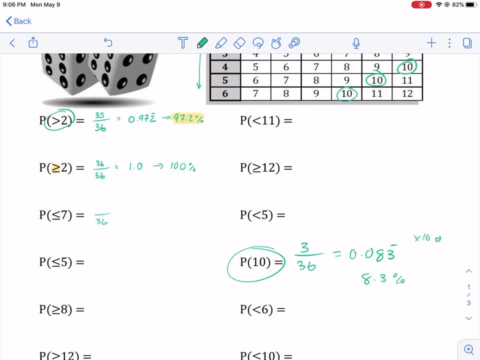 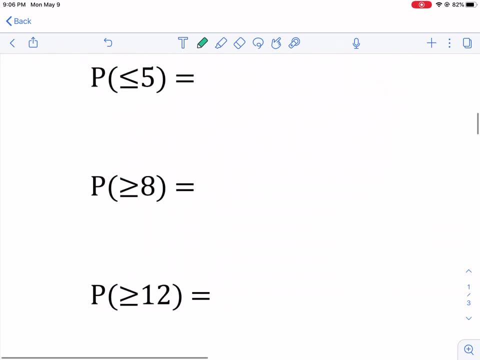 it into a percentage, as a reminder, you just multiply by a hundred or move the decimal place over two times 8.3%, And that's what you're doing with all of these. The important thing to know is if you're including the number. 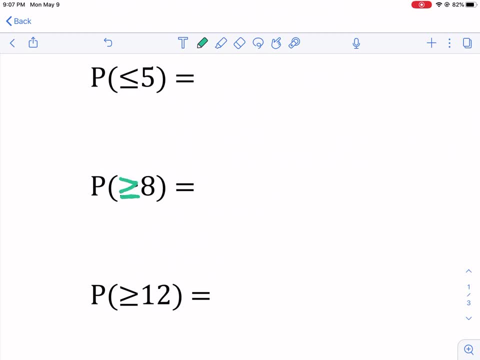 there's going to be this sign: the less than or greater than or sorry, greater than or equal to, or less than or equal to sign, And if it doesn't, it's just going to be without the line. So this is an example that you do not include that five. So you're just looking at all the values. 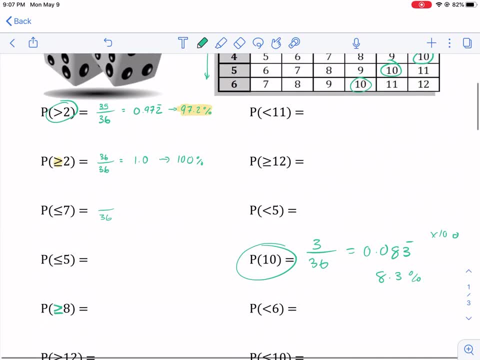 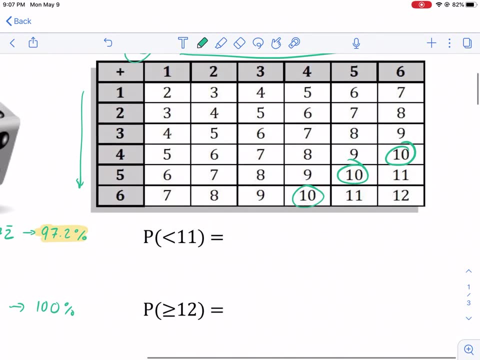 bigger than five. Okay, Seven's a big number here because it's most popular, So let's go ahead and do. P is less than or equal to seven. How many sevens are there? There's one, two, three, four. 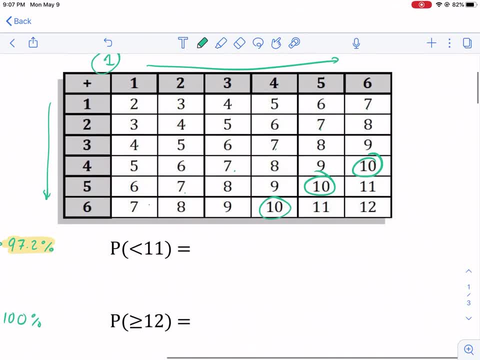 five, six, sevens, Okay, And I'm talking about less than so. I also need to talk about all these ones: One, two, three, four, five. Now I'm counting it as an aggregate, So I need to just add it to the six, So that's 11,, 12,, 13,, 14,, 15,, 16,, 17,, 18,, 19,. 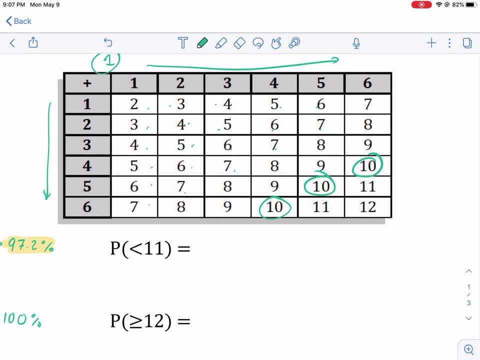 20,, 21.. That's how I would do it. You can also count the blank spaces and then subtract it from 36.. You'd count these guys. since they're bigger than seven, just subtract from 36.. But I just went ahead and did the other way. Okay, So again, that was six plus five is 11 plus four is 15,. 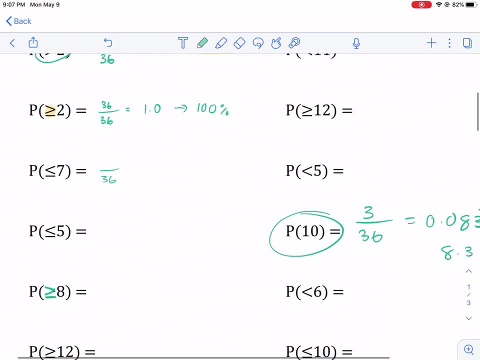 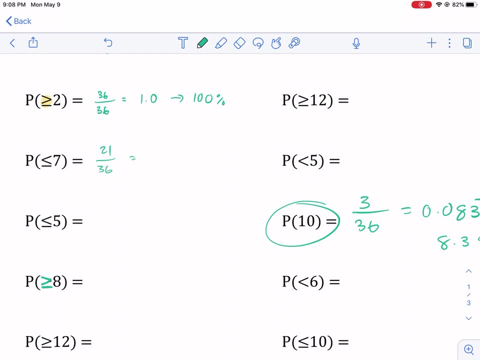 18, 20, 21.. Okay, So I have 21 out of 36 that are less than or equal to seven, 21 divided by 36.. And that gives me 0.583, or about 58.3% percent. Okay, And, as you can see, it looks like more than half of the. 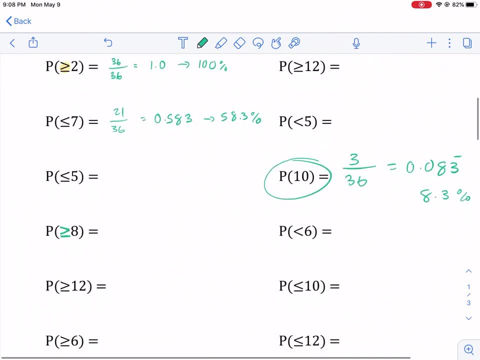 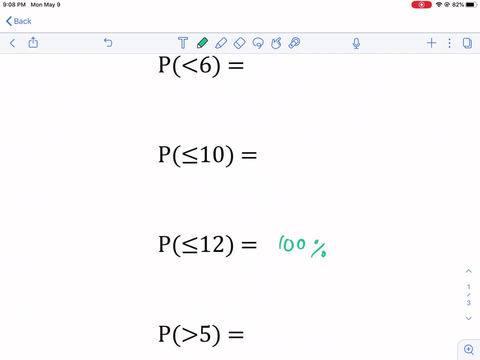 numbers, and it is okay, And that's it. That's all there is to it. So, if you want to, you know, help on any of these other ones. this one's going to be a hundred percent spoiler alert. Okay, We're talking about less than or equal to 12.. Well, that's all of them. 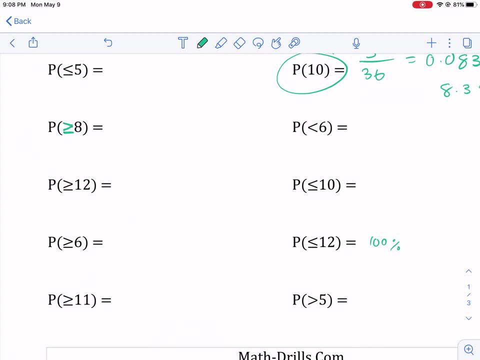 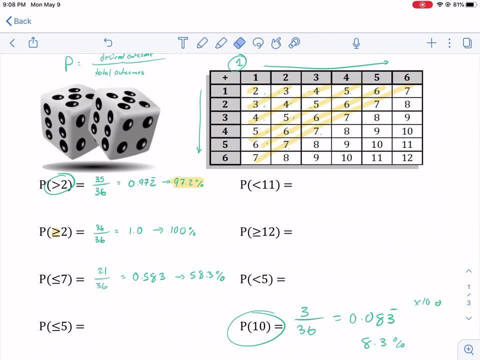 That's a hundred percent. but all these are going to be pretty, you know, pretty similar. This greater than or equal to 11, that's actually going to be a pretty small number greater than or equal to 11.. That's just going to be three numbers right here, And we already calculated. 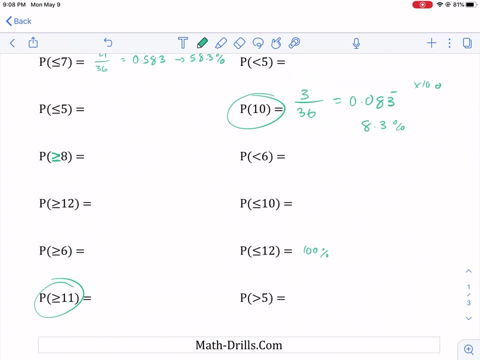 that Actually, we did this three out of 36, it's going to be the same percentage, So this is going to be 8.3%. So just make sure you're working smarter, not harder on this, but it's not much.